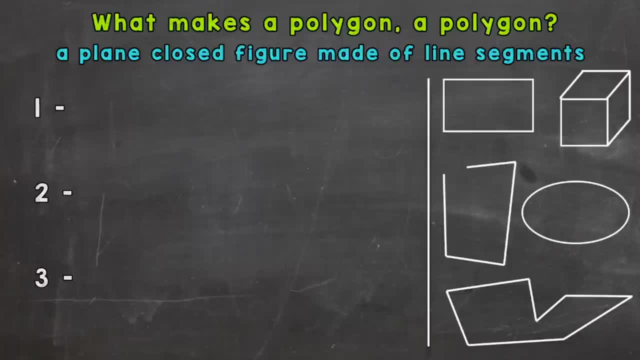 a three-sided polygon is a triangle. A four-sided polygon would be a quadrilateral. I'm going to go through those specific names in another video. I dropped that link that I put in the description, So I'm going to go through those specific names in another video. 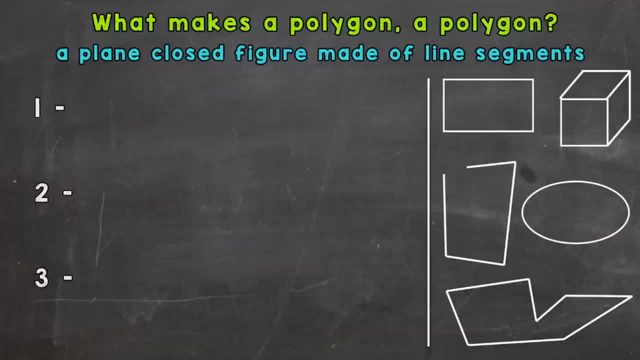 So let's get back to what makes a polygon a polygon. So the first characteristic or thing in our checklist: a plain figure or plain shape. That just means the figure or shape has to be flat. So if it's three-dimensional, like a cube, a pyramid, a rectangular prism, 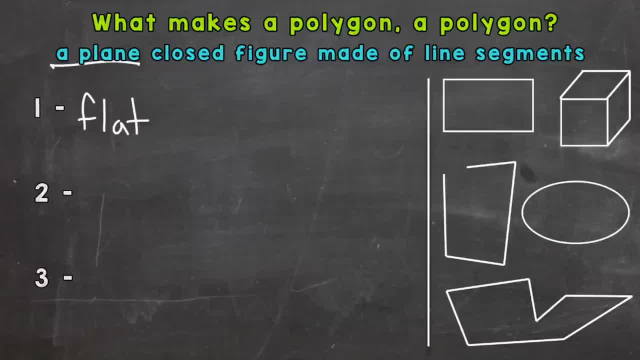 those are not polygons. So again, has to be flat. Next closed. So a closed figure or shape, And that's exactly what it sounds like. It has to be closed. So I will give you a counter example. that's not a polygon. So let's say we almost have a rectangle. 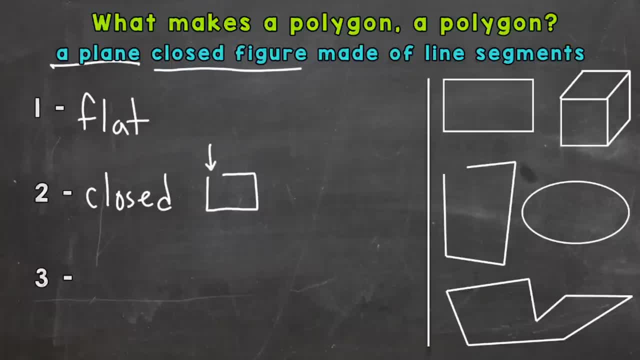 here, but we have this opening. That would not be a polygon, because it's not closed, So not a polygon. And then, lastly, it's made of line segments, So I'll put line segments here. This means that there cannot be any rounded edges. So, for example, actually a counter example- 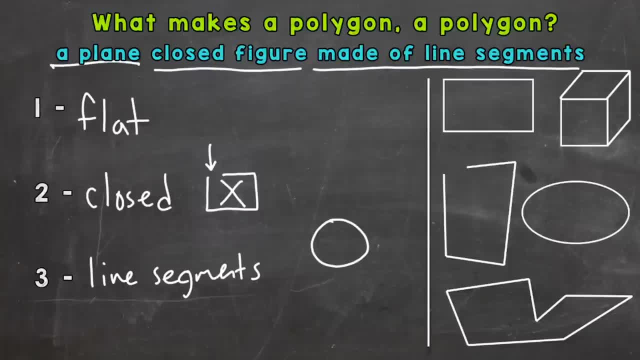 a circle is not a polygon. Yes, it's flat, Yes it's closed, but it's not made of line segments. A polygon has to have a check next to each of these three things, So not a polygon. Another counter example would be a figure like this: It's looking like it will be a rectangle. 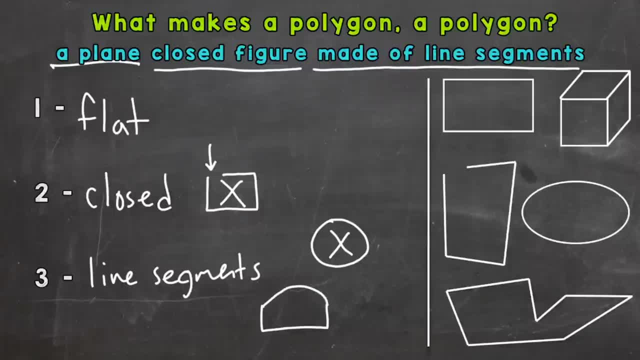 but we have a rounded top here, So not a polygon, because it's not made of all line segments. So let's take a look at the right hand side of your screen. here We're going to go through five different figures and determine if they are polygons. So the first one here: